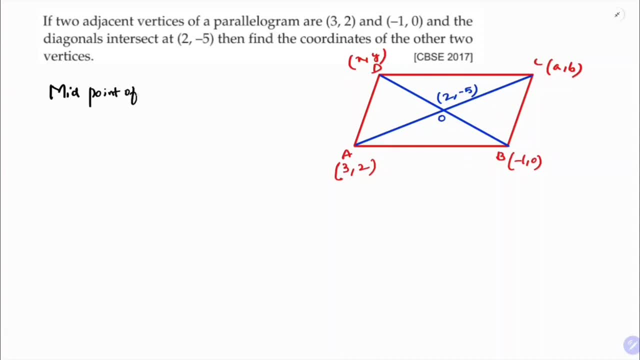 given Midpoint of AC is given. Midpoint of AC is given. So midpoint of A, 3 comma 2, C, A comma B is 2 comma minus 5.. So midpoint formula is X1 plus X2 by 2, Y1 plus Y2 by 2, is 2 comma minus 5, because in 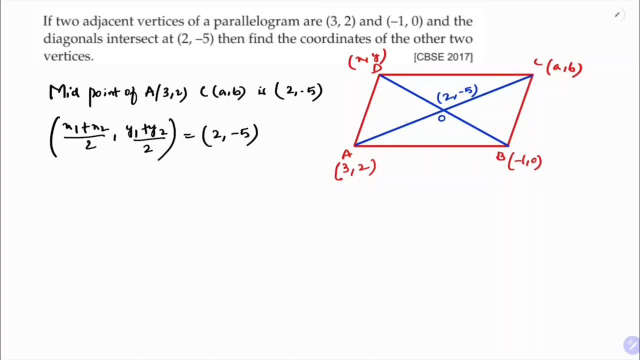 a parallelogram, diagonals bisect each other means where the diagonals will meet, they'll bisect each other at that point. So midpoint of AC is 2 comma minus 5 and midpoint of BD is also 2 comma minus 5. 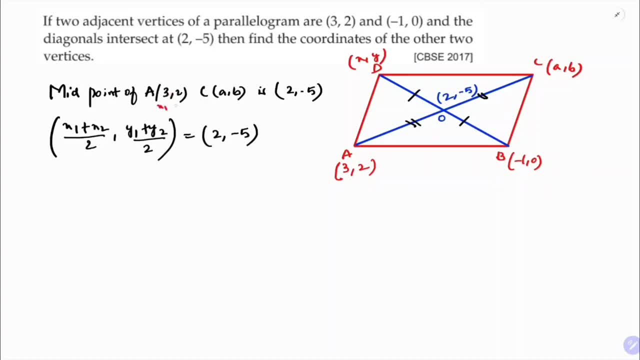 so now, if I substitute the values here x1, y1, x2, y2, so 3 plus a by 2, 2 plus b by 2 is 2 comma minus 5. so now, if I equate abscissa with abscissa and ordinate with ordinate, 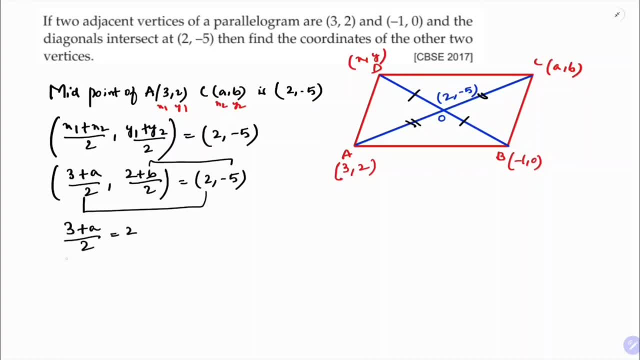 so 3 plus a by 2 is 2. 3 plus a equals 4, because 2 times 2. so a is 4 minus 3, so the value of a is 1. next one: if I equate ordinate with ordinate, 2 plus b by 2 is minus 5, 2 plus b. 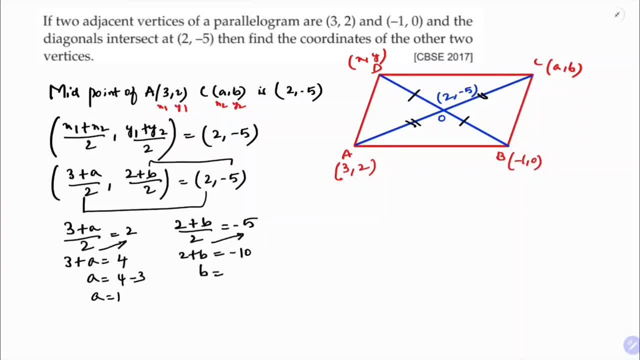 equals minus 10, because 2 times minus 5, minus 10 and plus 2. if I transpose minus 2, so b value is minus 12. so the vertex c is a comma b, which is nothing but 1 comma minus 12. in the same way, now, midpoint of midpoint of b and d, midpoint of b and d. 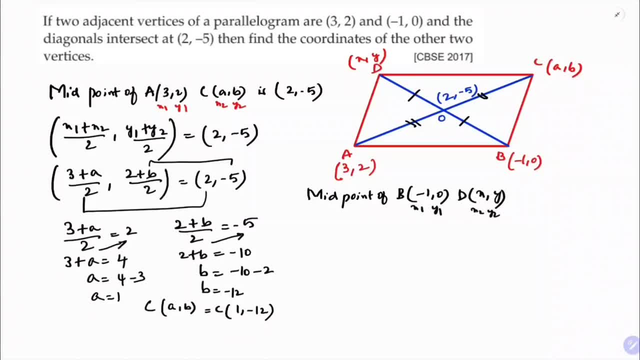 is also 2 comma minus 5. x1 plus x2 by 2, y1 plus y2 by 2 is 2 comma minus 5. so if I equate abscissa with abscissa here, 1 plus x by 2 is 2, 0 plus y, is y by 2 equals minus 5. so